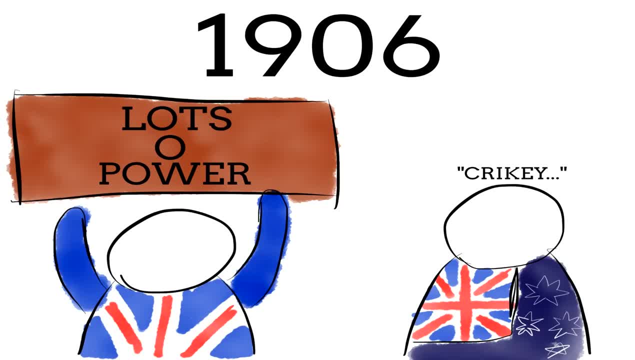 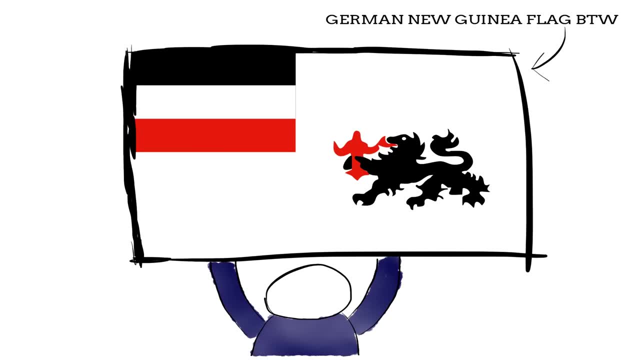 Australia and in 1906 gave the rest of their power over the land to Australia, and British New Guinea became the territory of Papua. Then again, during World War one, Australian forces seized German New Guinea, which eventually became the territory of New Guinea, Collectively the eastern part of the. 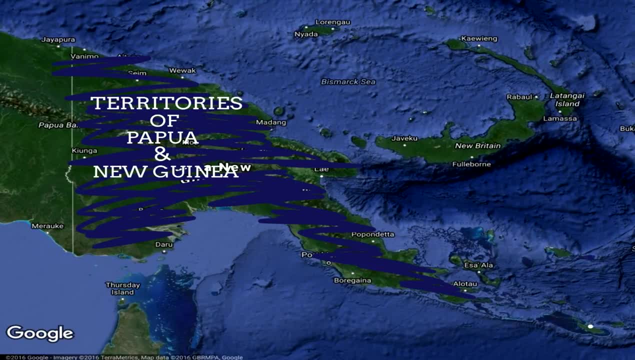 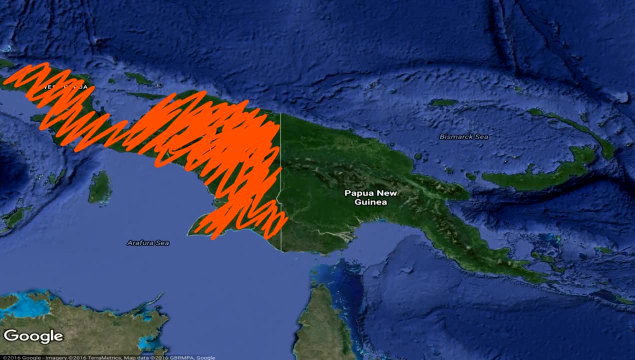 island claimed by Australia became known as the territories of Papua and New Guinea. Man, those Australians really wanted that island. So by the 1920s we have the west of the island under Dutch control and the east of the island under Australian control. Yet with foresight on our side, we know things don't stay. that way. First off, in the west, with Netherlands, New Guinea, their closest country neighbor Indonesia, which had earlier become an independent nation breaking free from Dutch control, wanted to claim that land as their own. They launched an attack against the territory, which didn't go too well, Yet, despite a 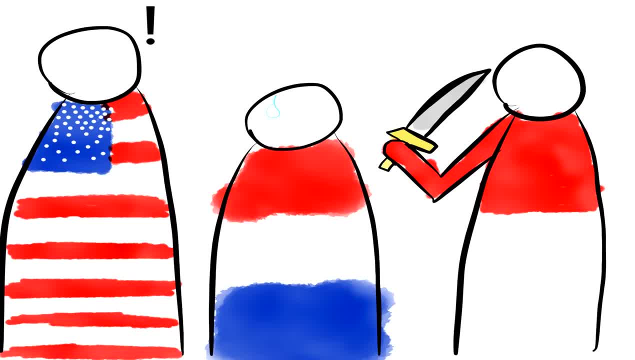 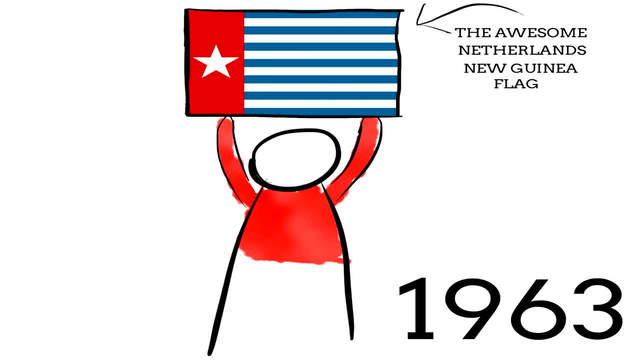 loss, pressure from the United States and fear that the Indonesians would invade again. the Dutch agreed to re-enter negotiations and, after a lot of dull talking, the land was given to Indonesia in 1964.. On the Australian side, however, things aren't quite as exciting. No war, no. 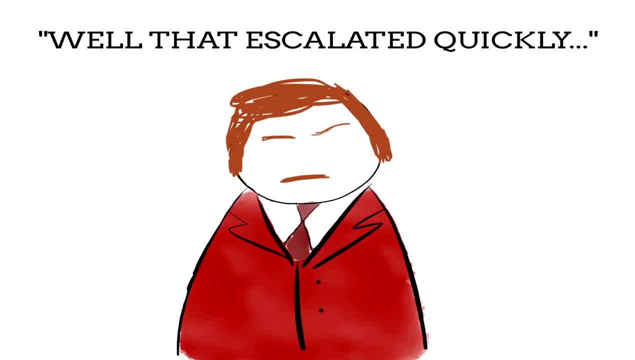 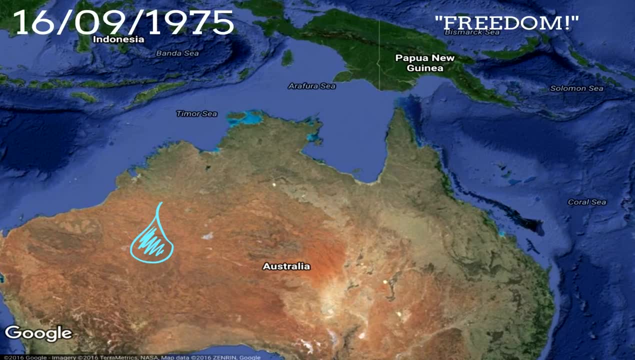 pressure. no, Dutch, It kind of just happened really. The land eventually became known as Papua New Guinea. It became self-governed in 1973 and achieved independence from Australia on the 16th of September 1975.. This is how. 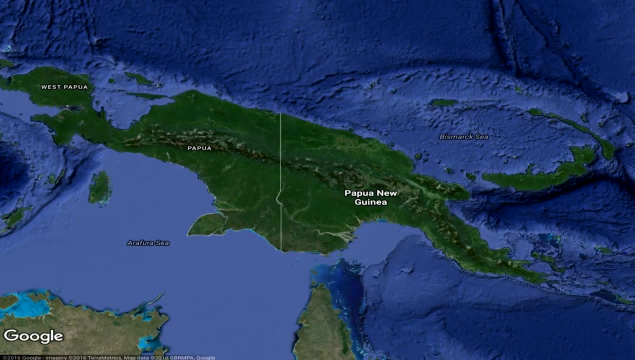 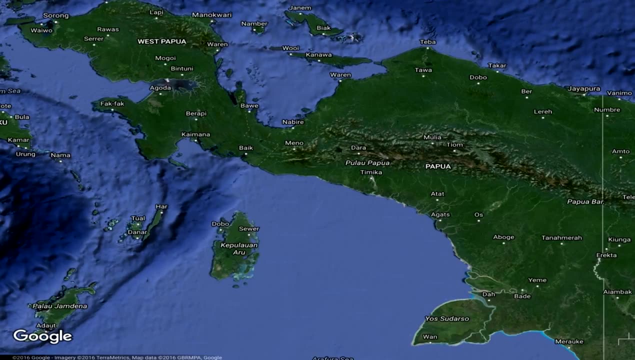 the island is split to this very day, except there's a tad more to it than just separate country in the east and region of Indonesia in the west, For the region of the island that belongs to Indonesia is actually split a further time To two separate provinces: Papua and West Papua. Not only that, but the country of 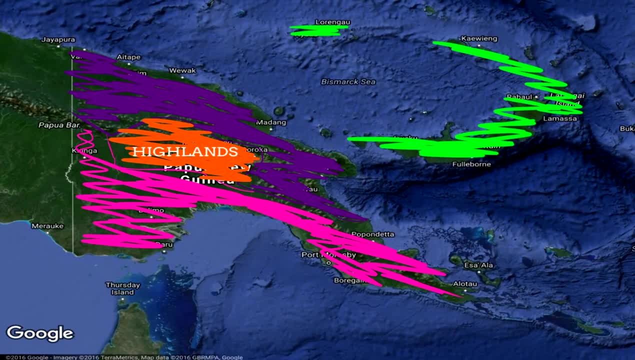 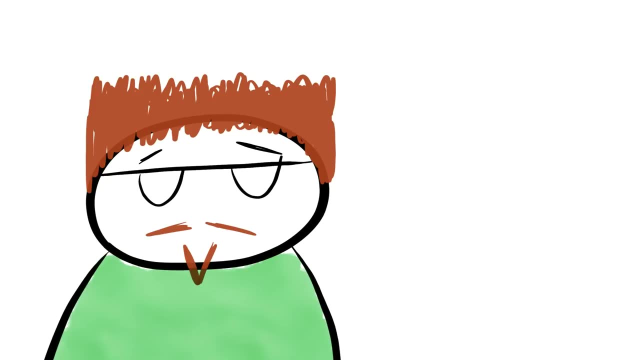 Papua New Guinea is, too, split into four regions: The Highland region, the island region, the Mamasi region and, yes, of course, the Papua region. And, yes, each of these regions in turn split into smaller provinces, but let's not talk about those. So we have one island that consists, on the east, of four regions that create a 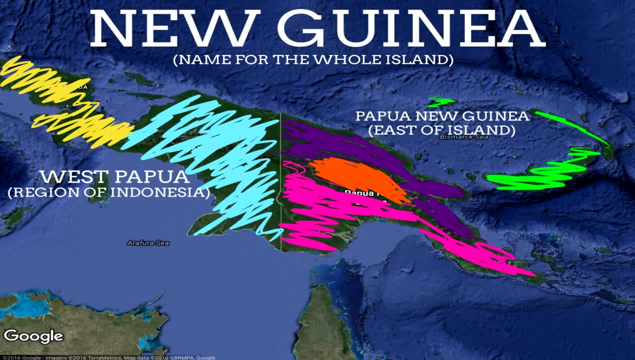 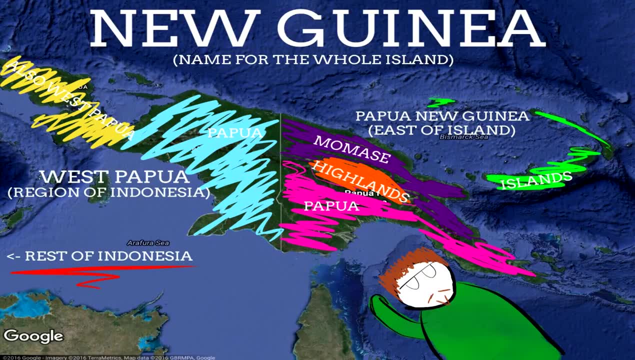 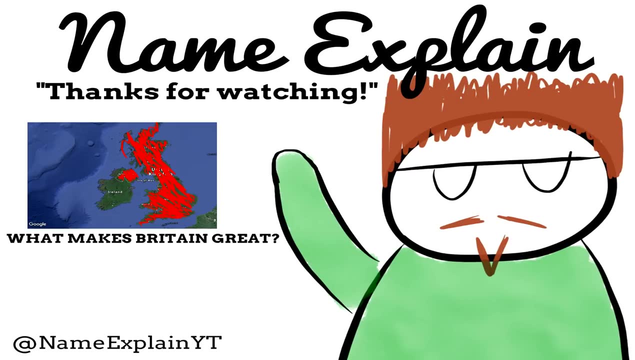 whole country and, on the west, two provinces that create one region that adds to one whole country, Giving us a lot of interesting names and a very interesting story. Well, I think so, anyway. Papua, Papua, Papua, Papa, I don't know, Tell me in the comments if I've been wrong saying that word.